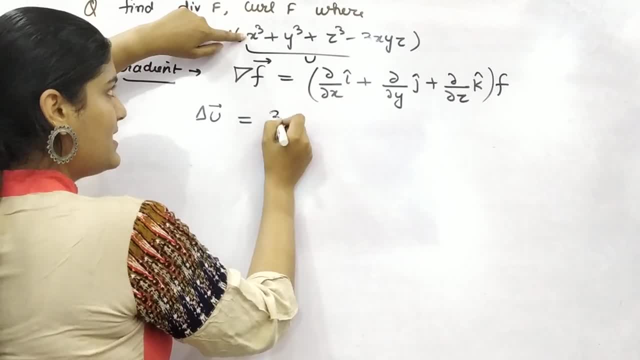 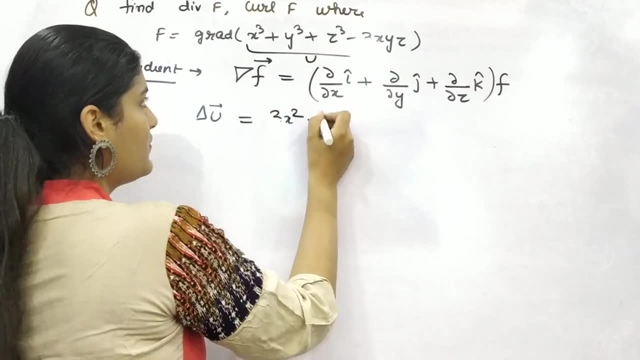 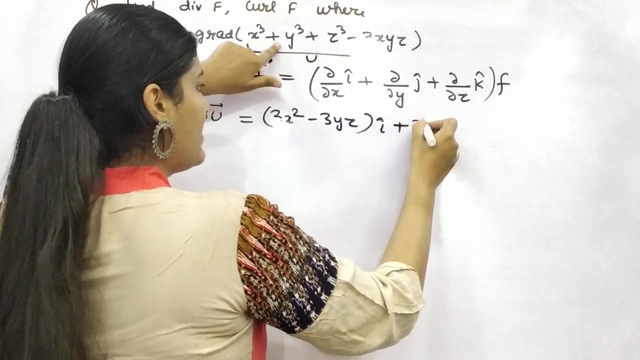 to x in x direction, right? So this is 3x square differentiation, because you are keeping y and z constant, so 0 and this will be 3yz. okay, In i direction. then, with respect to y, 3y square minus 3xz, with respect to, along with: 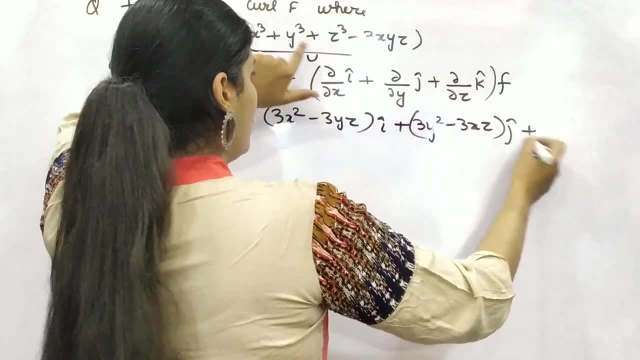 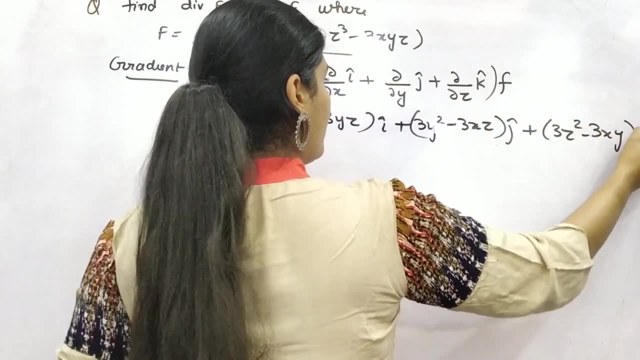 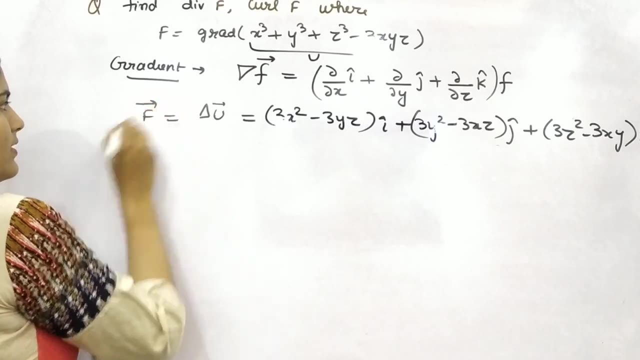 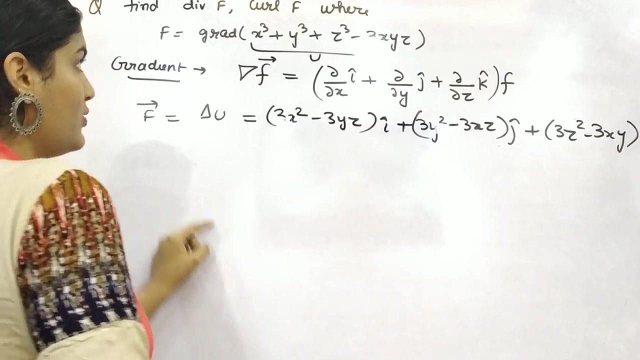 y axis and thereafter, when you will differentiate it with respect to z, you will get 3z square minus 3xy. okay, alright, So this is your f correct. You have got your gradient now. this is your f function. Now you have to find out divergence. 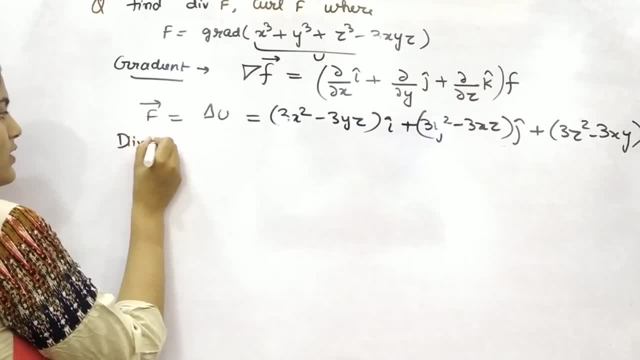 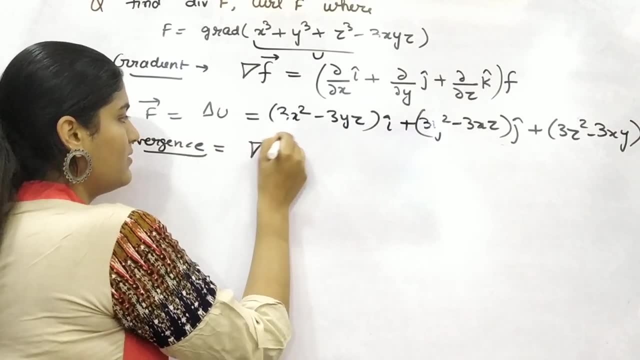 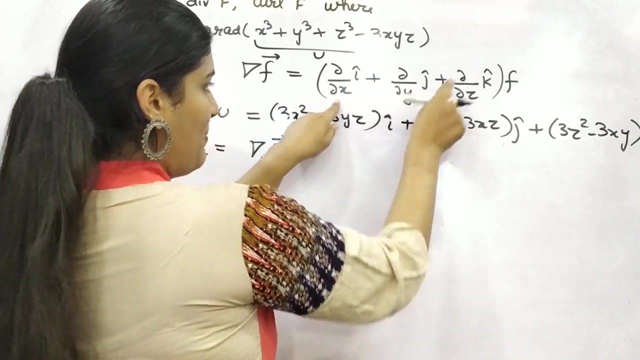 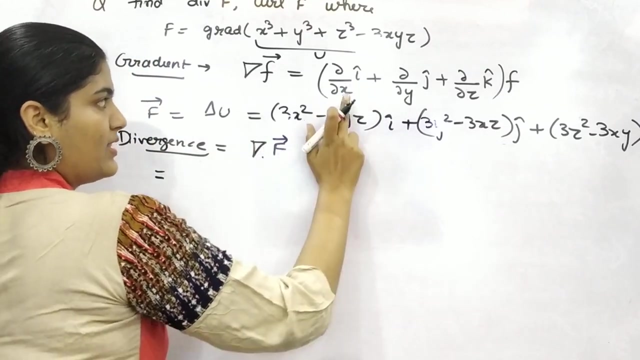 of f. So how can you calculate it? So divergence is gradient of that particular function. okay, So that means you need to apply this formula. and now your function is this: alright, So iz is the z axis and this is the z axis, so you just need to take the f. okay, If you? 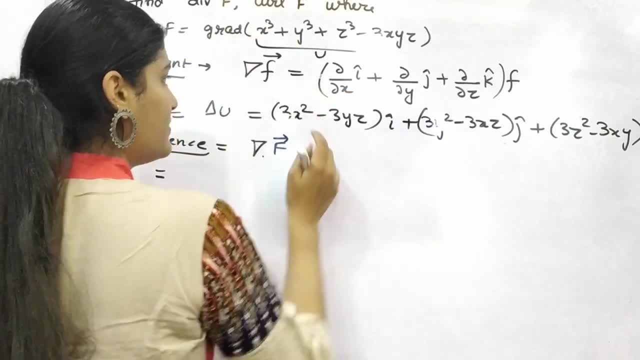 want to do that, take the z axis, so you will find that let me do it here. iz is the z axis and then iz is the z axis because it is the z axis. Okay, so you can do this by. 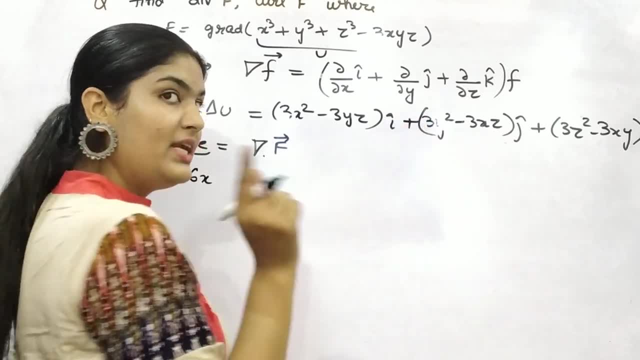 taking the f of i, so iz is the z axis and then the x is the x axis. Okay, so this is what you will get. this is the y axis And you will also do the dy with respect to x. 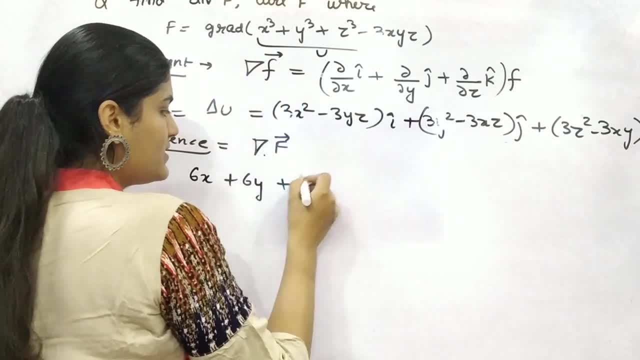 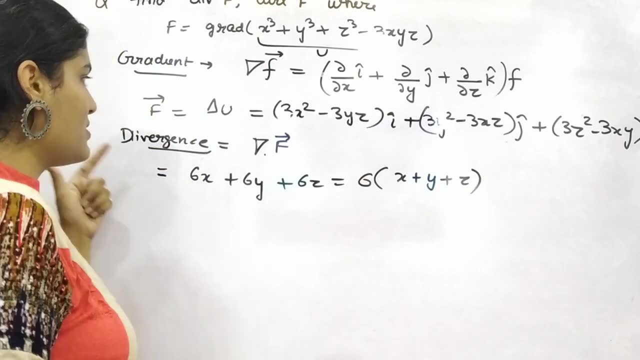 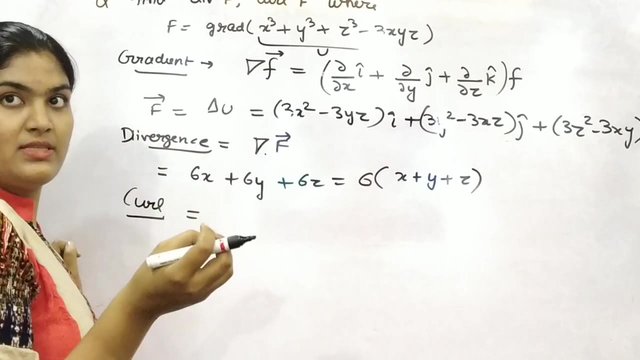 oh, it's the same function again, right? So you will find that if you do this property common, Okay, so this is your divergence. Now, in order to find out curl, there is slight difference between divergence and curl. Divergence is dot product and curl is cross product. 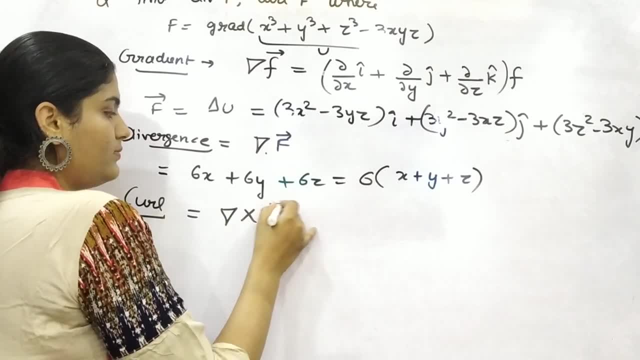 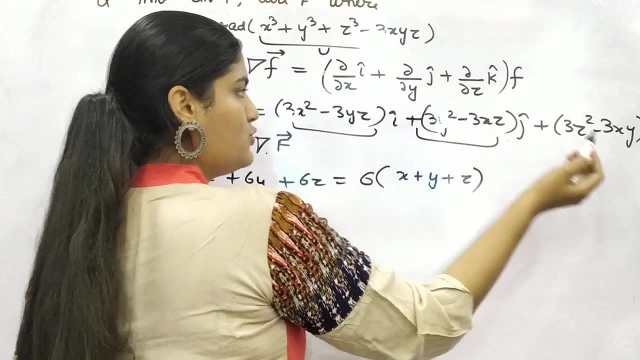 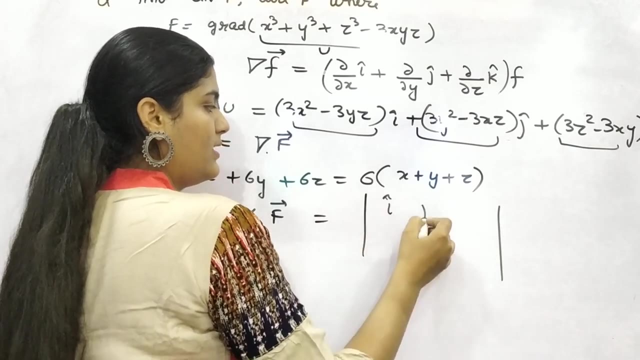 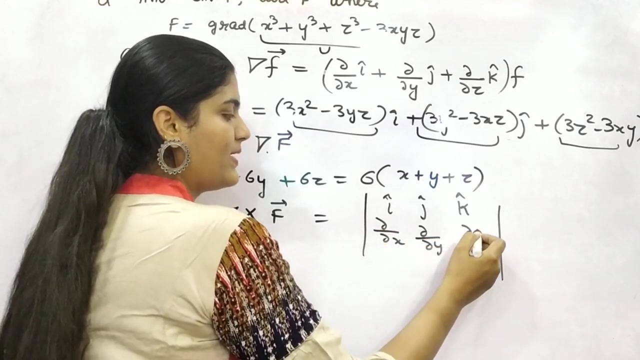 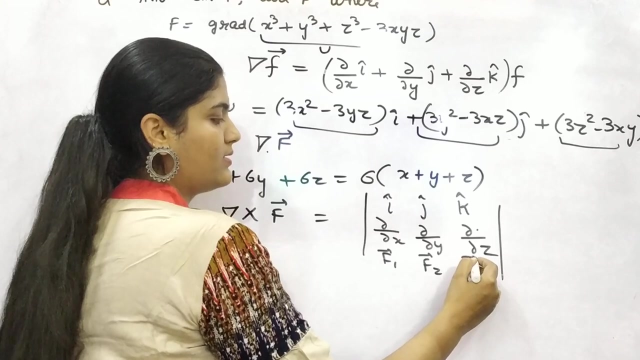 What is it Cross? You can see that your function is divided into three parts. Let's say f1, f2 and f3.. So your cross product will be like: i, j, k, partial differentiation with respect to x, with respect to y, with respect to z, with f1, f2 and f3 parts. Okay, so let's. 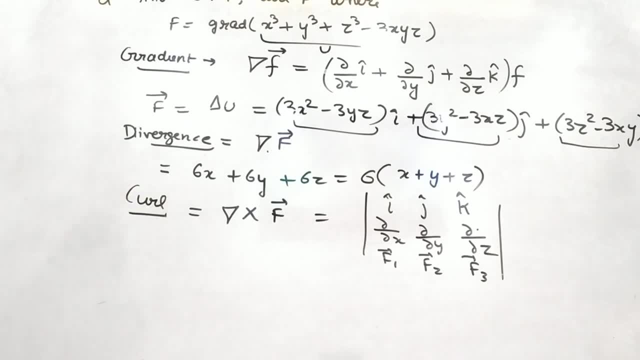 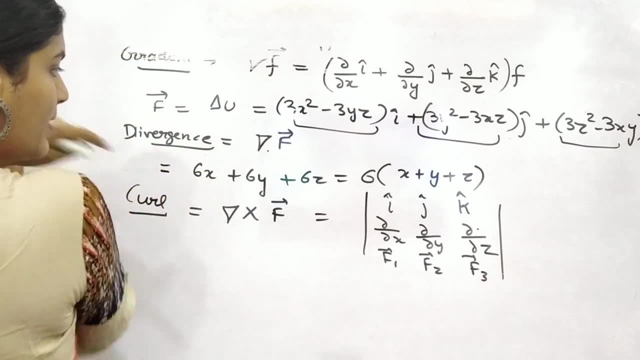 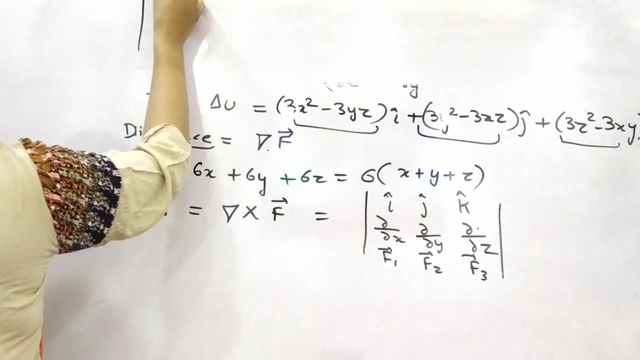 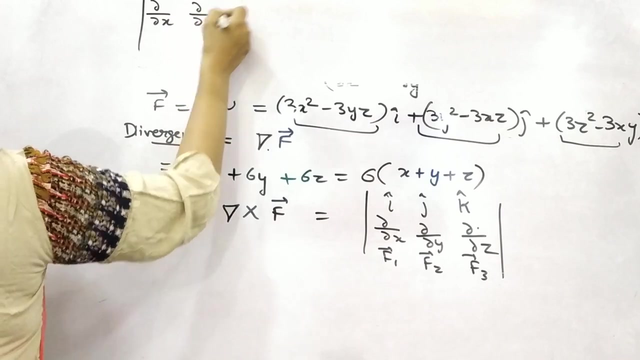 apply this formula using these values. Okay, let me grab adjuster. So, because you are using this bit so I cannot erase it, Let me write it first. So your i, j, k. Okay, then, after partial differentiation, with respect to x, with respect to y, with: 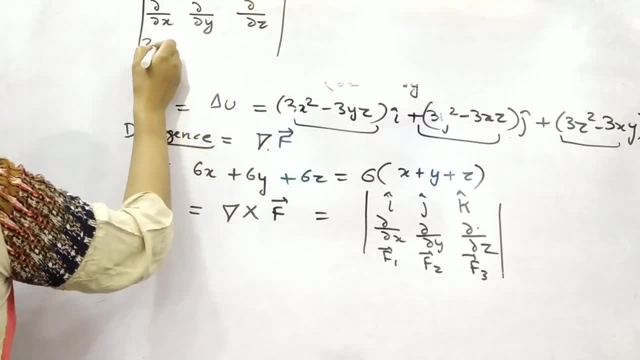 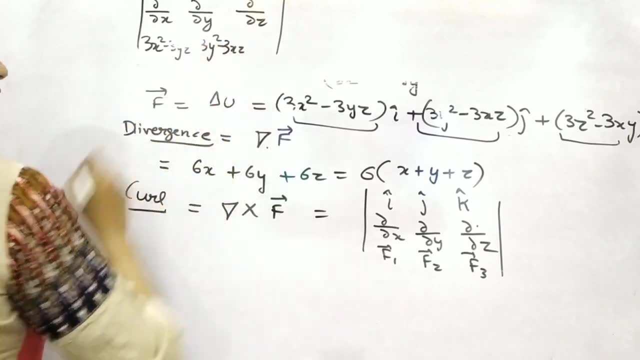 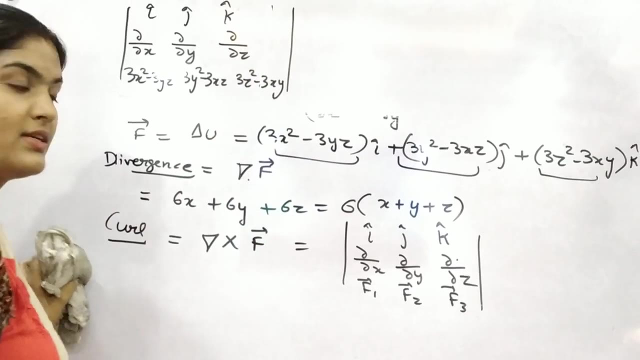 respect to z, your first part is 3x square minus 3yz. Your second part is 3y square minus 3xz And third part is 3z square minus 3xy. Correct, Let me erase it now. So if you solve this, 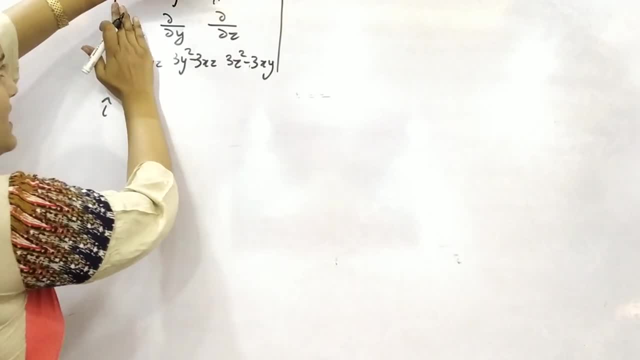 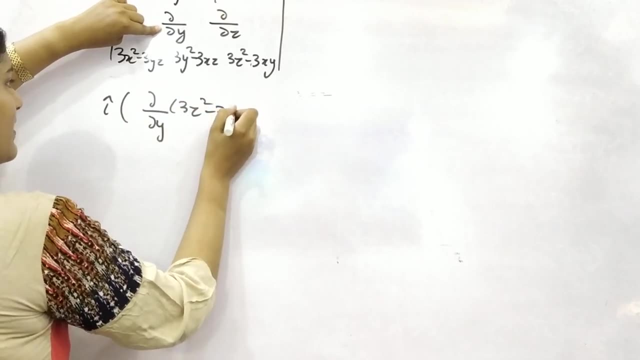 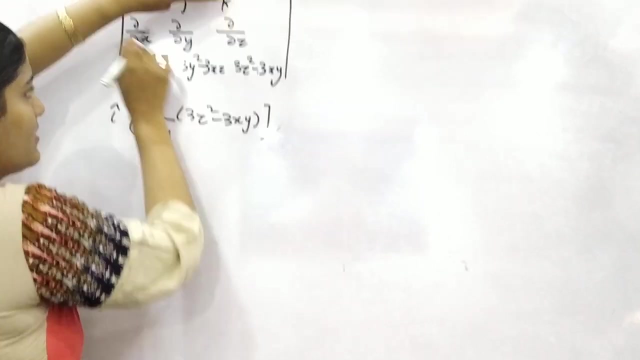 you know how to solve determinant right, I erase it and this will be differentiation of this bit: 3z square minus 3xy, right After minus j. sorry, So you are hiding this. This multiplied this minus minus is in formula this way You are. 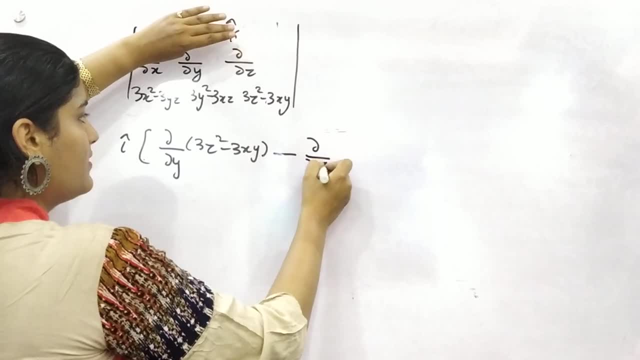 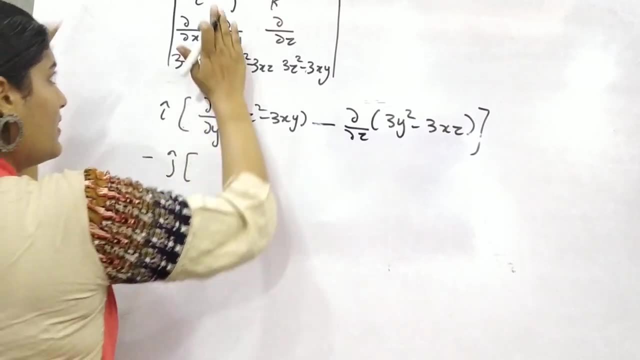 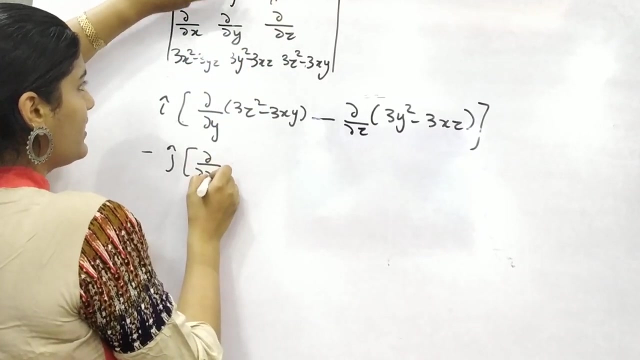 hiding this. So this multiplied this and this multiplied this right. Then after minus, is in formula: Hide the row of j and column of j. What you get Differentiation with respect to x of this part: 3z square minus 3xy. 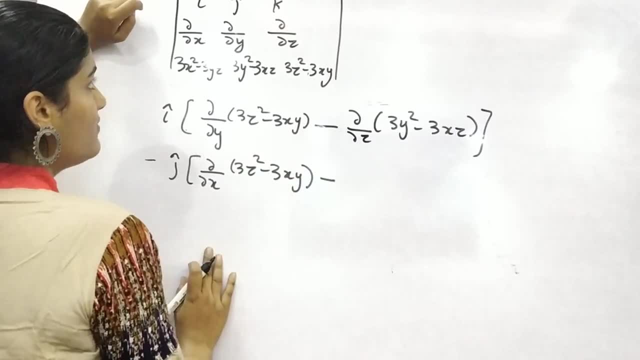 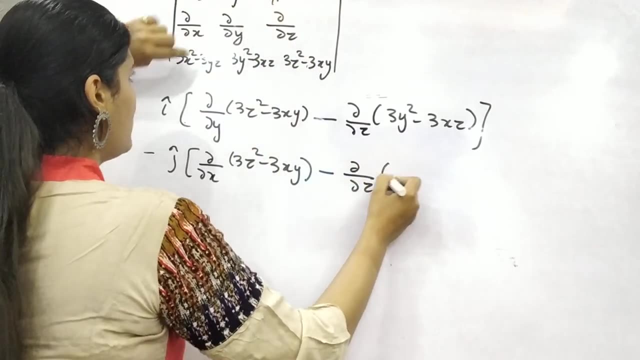 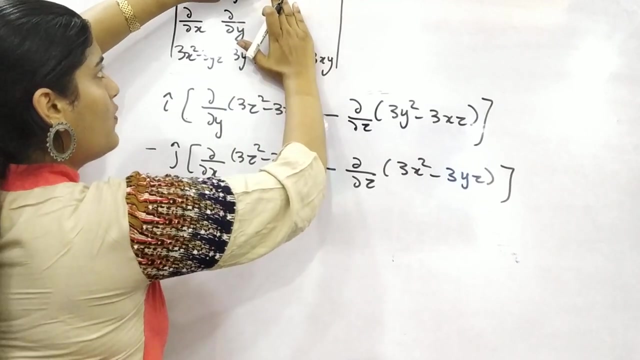 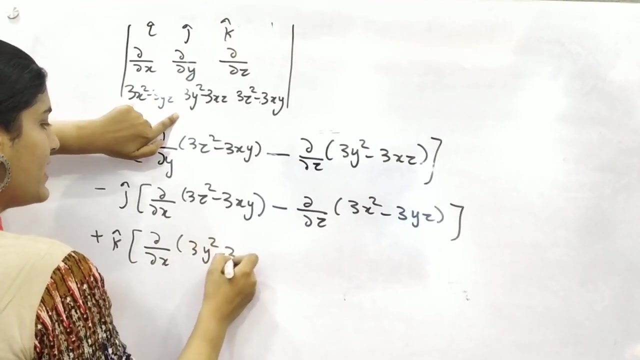 Okay, Okay, Minus is in formula. You are hiding j. This bit is solved Now, minus differentiation with respect to z of this part. Thereafter k hide the row and column in which k exists. So differentiation of 3y square minus 3xz minus differentiation 3x square minus 3yz. 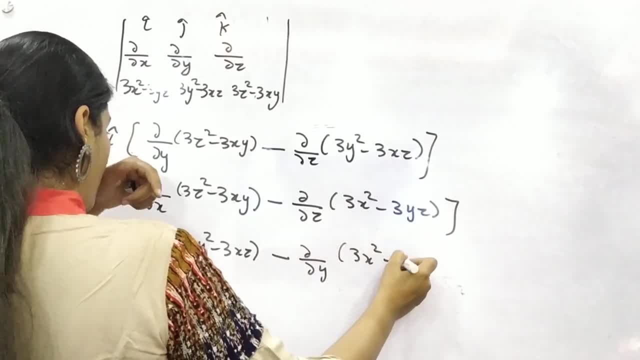 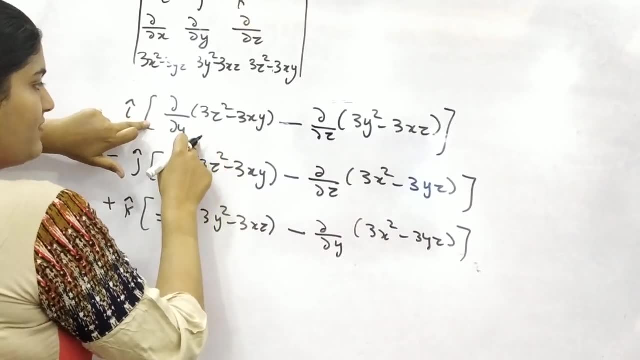 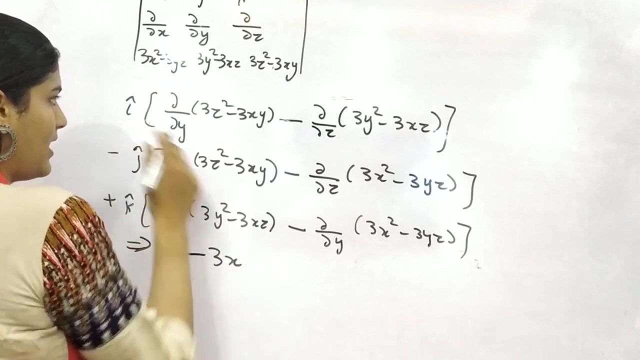 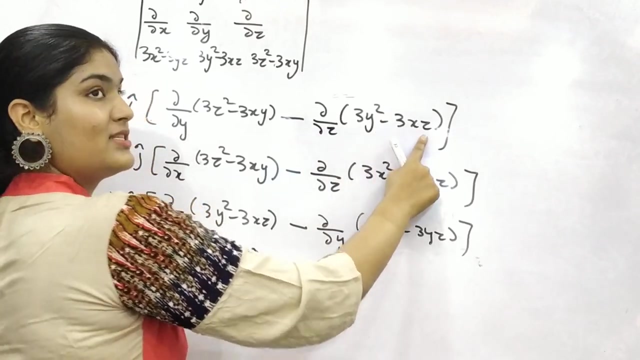 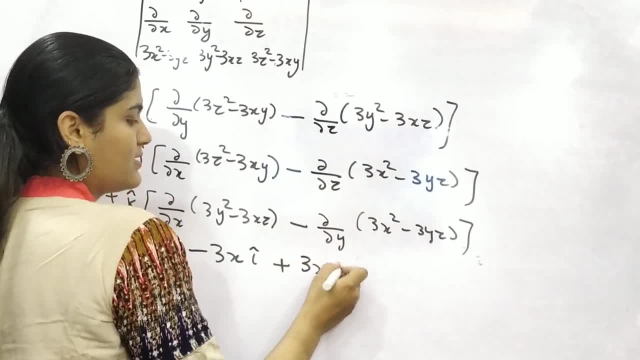 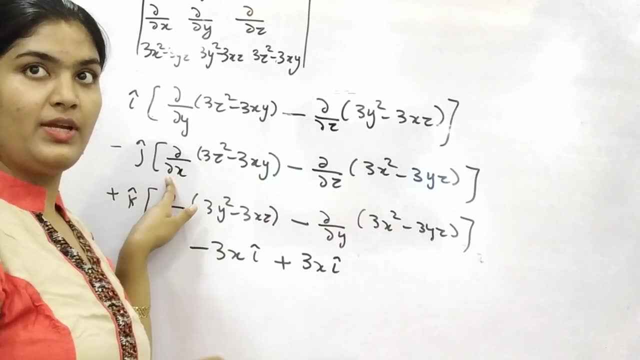 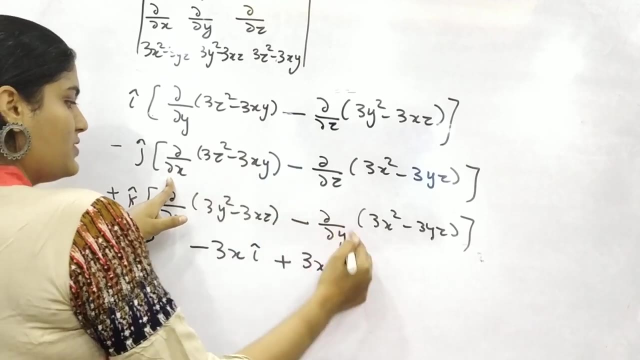 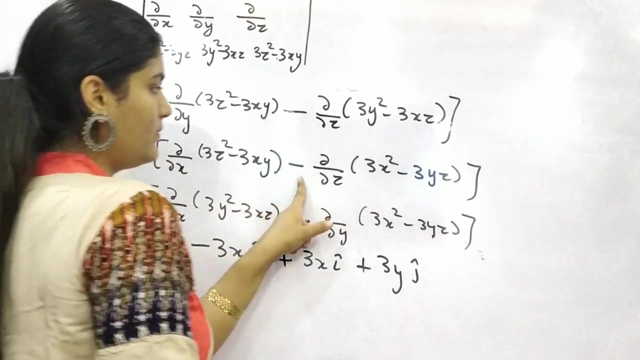 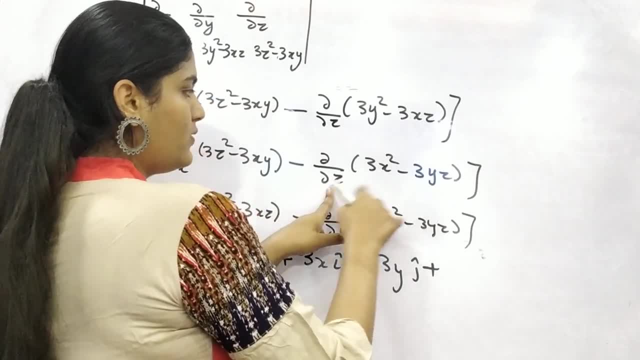 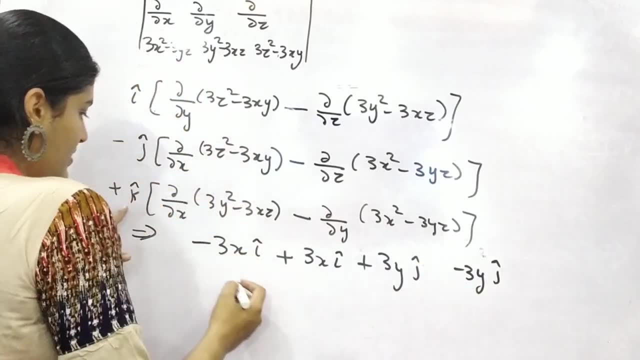 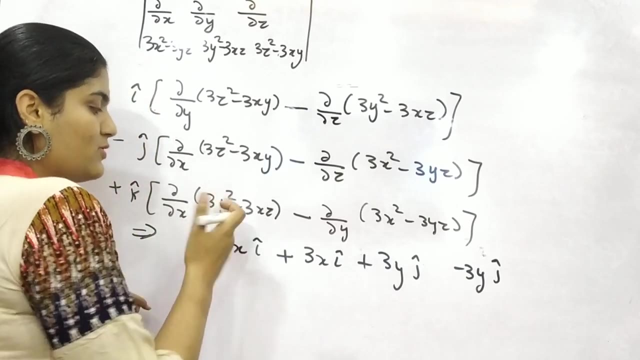 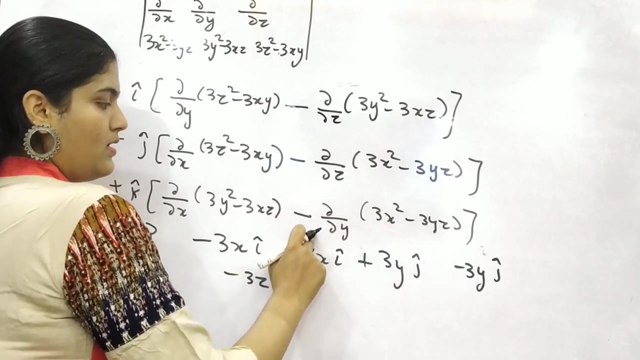 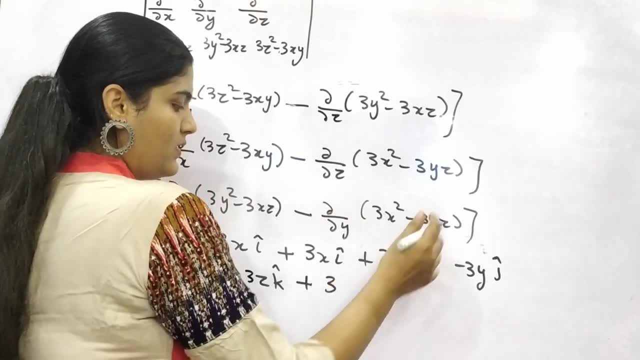 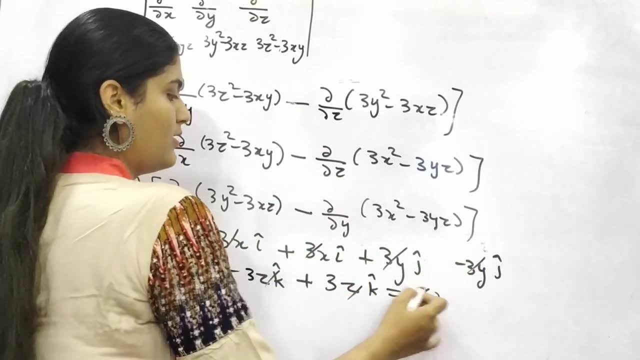 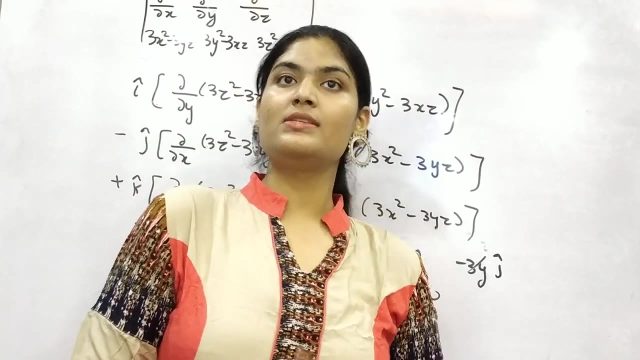 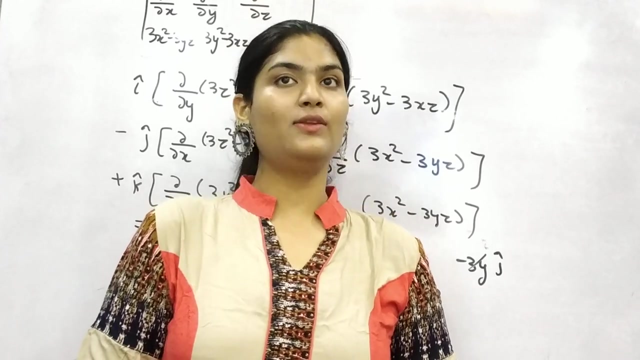